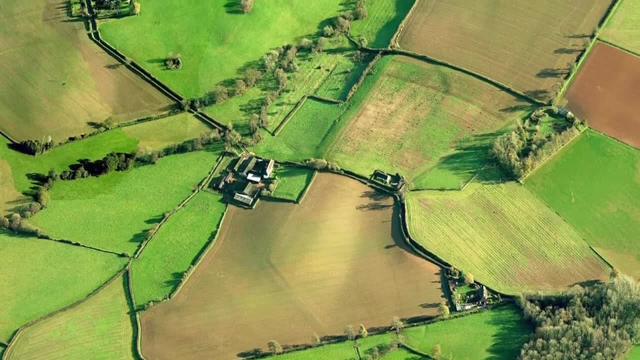 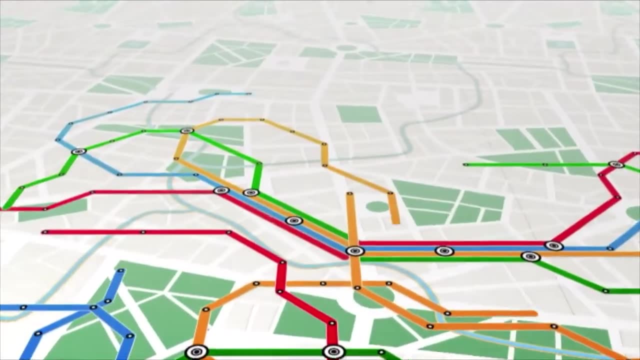 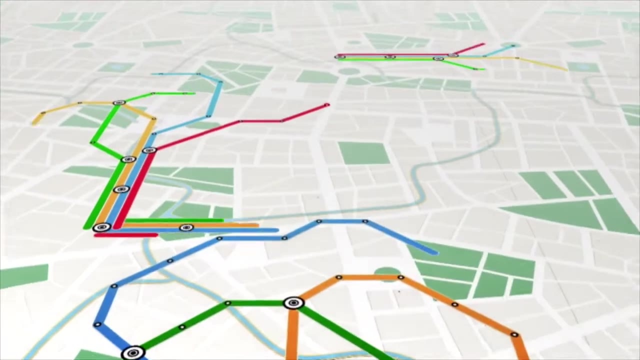 together. So how do we make sense of this hugely diverse and highly complex spatial information? Well, the first thing we do is to simplify the process by breaking the real world down into layers, Each layer which can represent point locations, areas or networks of lines. 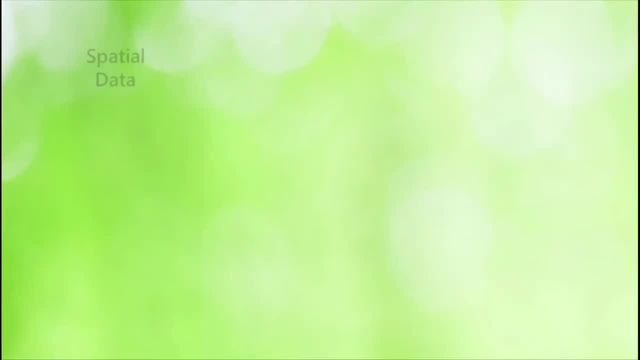 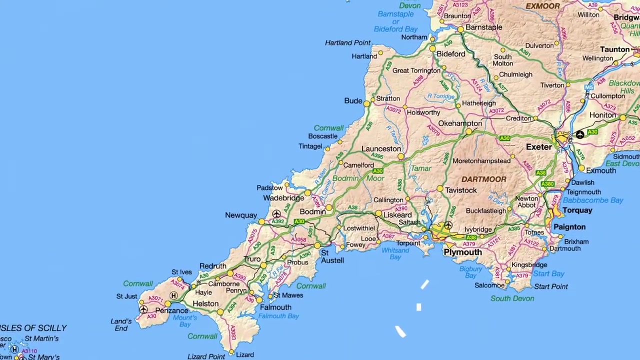 is used to represent just one set of features in our landscape. Once created, these layers of spatial data can then be combined together, interpreted, analysed or visualised to create the geographic information we need to make sense of the world around us. Take an ordnance survey map of South West Australia. 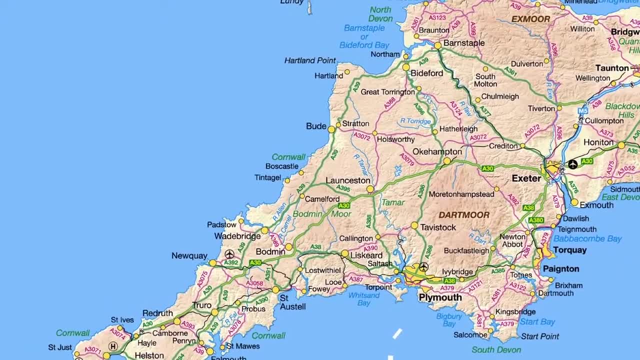 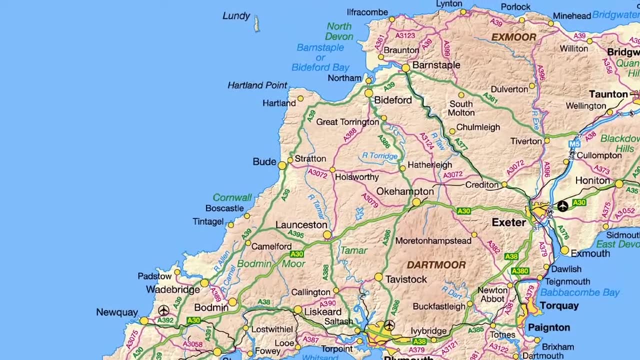 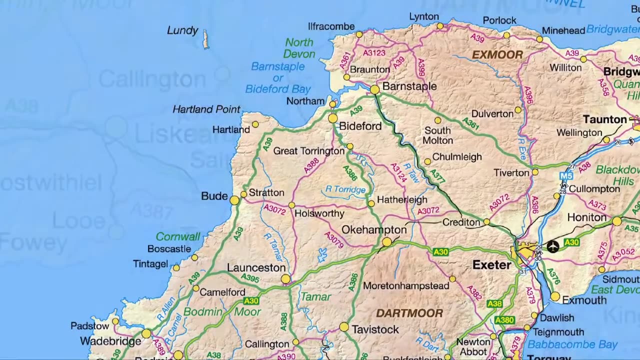 Even this simple map, which is designed to be used as a navigational aid, illustrates how complex the myriad of features in our landscape can become when they are overlaid. What's clever about this map is that, despite the complexity of the data shown by dividing 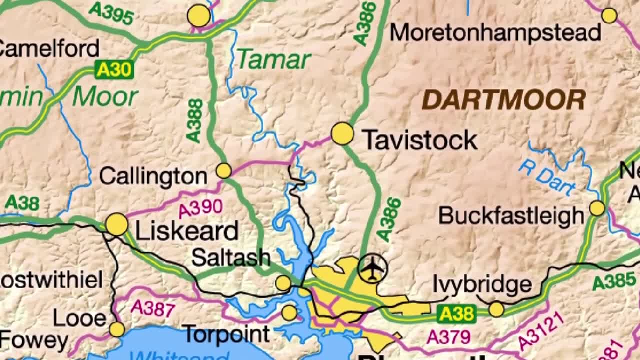 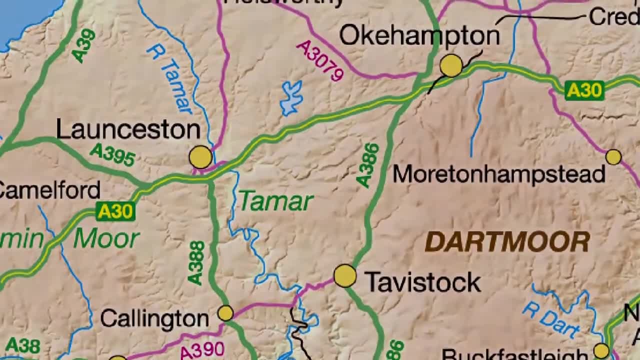 the features into different types and representing them in different ways, its creator has still managed to create a powerful, visually striking and easy to interpret piece of geographic information. So what's the point of creating a map of South West England So to understand our landscapes, how they work and, perhaps most importantly, how we? 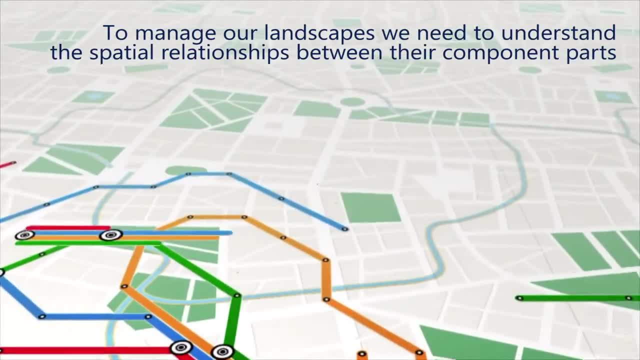 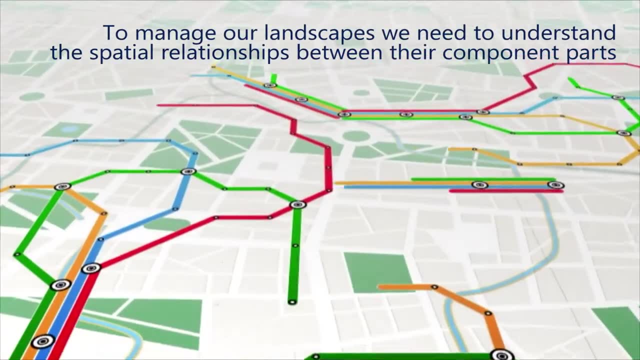 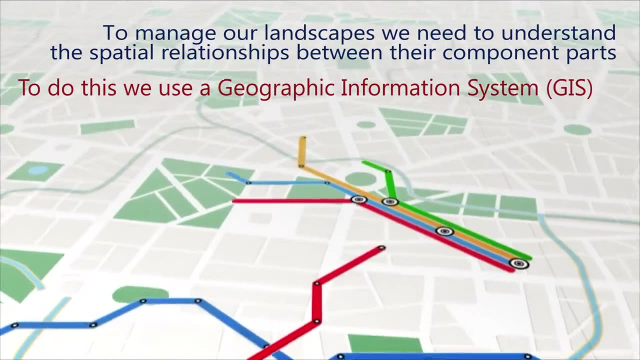 should manage them. we need a way to visualise and explore the spatial relationships between their different component parts and, in so doing, generate the geographic information that we need. The way we do this is to use a tool called a Geographic Information System, or GIS. 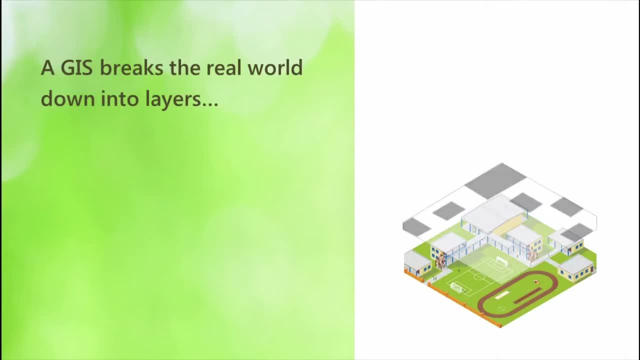 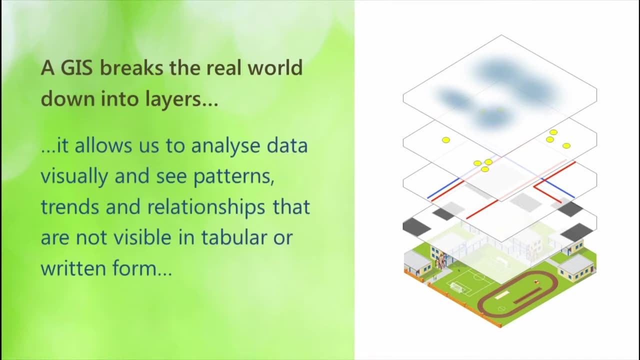 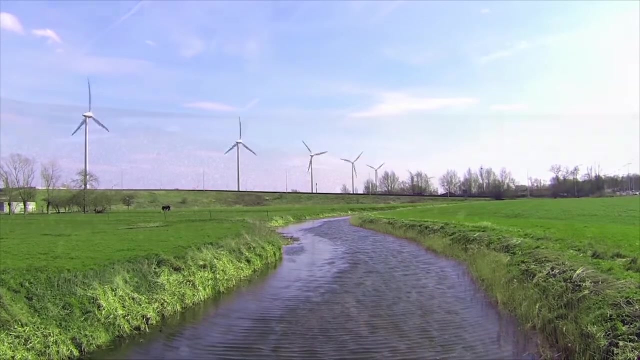 A GIS allows us to break the real world down into layers and, having done this, it then allows us to analyse data visually. This allows us to see patterns, trends and relationships that are not easily recognisable in a table or written as words. 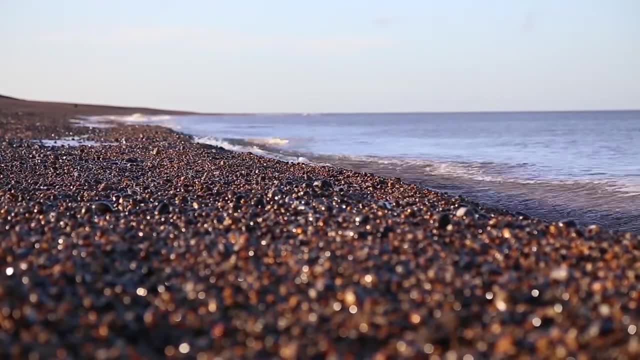 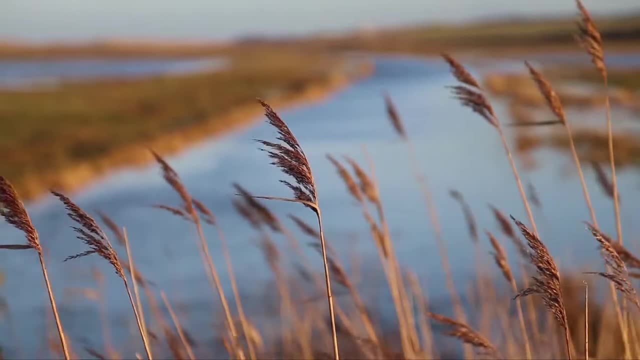 As an environmental professional, we will often visit a specific location- a river, a farm or a natural habitat- to study it. We want to learn about its character or its condition. We can actually learn a lot about a place by visiting it. 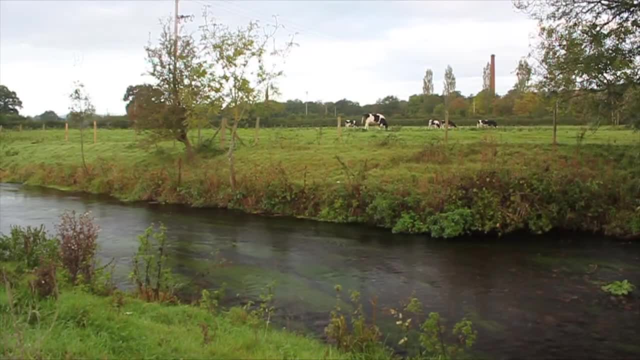 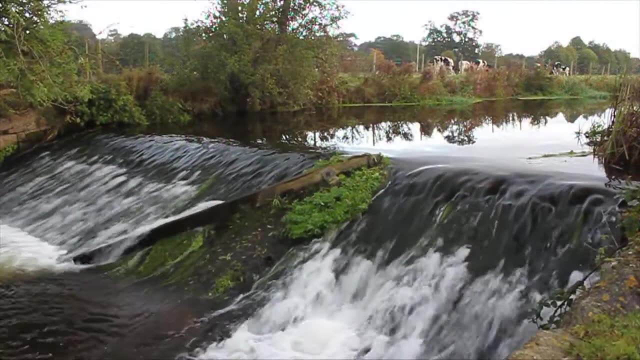 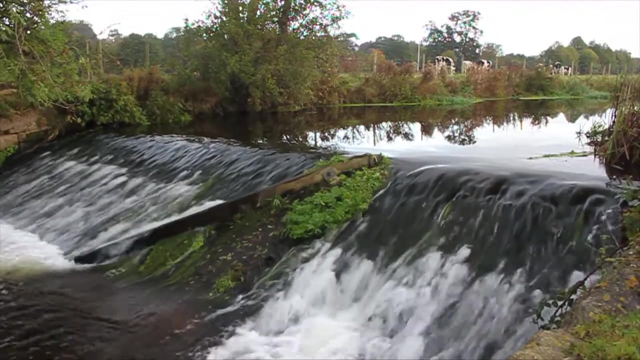 We can measure the chemical composition or physical properties of the environment, Or we can record the species that we observe or the structure of the surrounding habitat. But there are also many questions about a location that we cannot answer by simply going to it. For example, we can't see how it fits into the wider landscape. 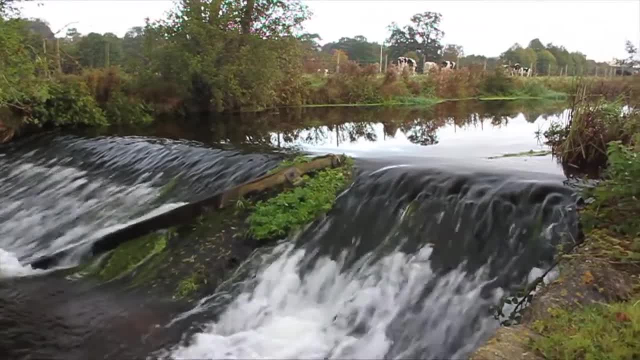 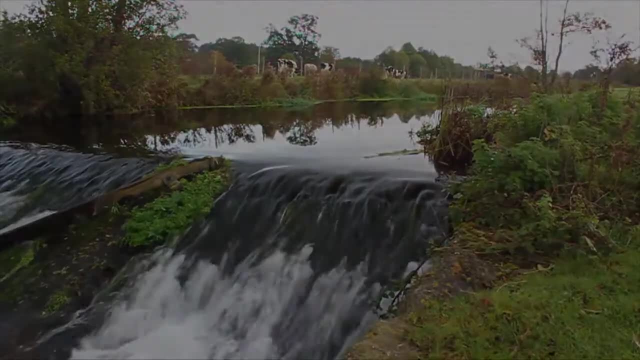 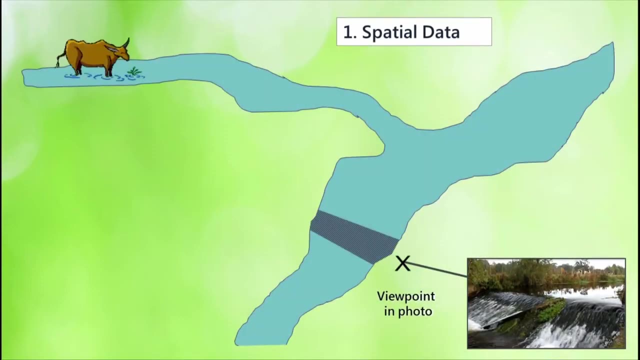 We can't see its size, its shape, We can't see the composition of the surrounding area And, perhaps most importantly, we can't see how it is connected to other similar locations nearby. Using a GIS, we can answer these questions. In a GIS, we create spatial data to graphically represent the features in the landscape. 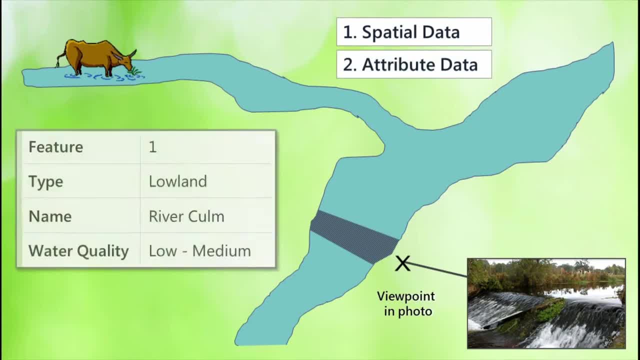 And then we can also record additional information about them, referred to as attributes. By placing the features into a measured grid, we can go further and determine the size, shape and orientation of the different elements. We can also begin to visualize how different elements of the landscape are connected together. 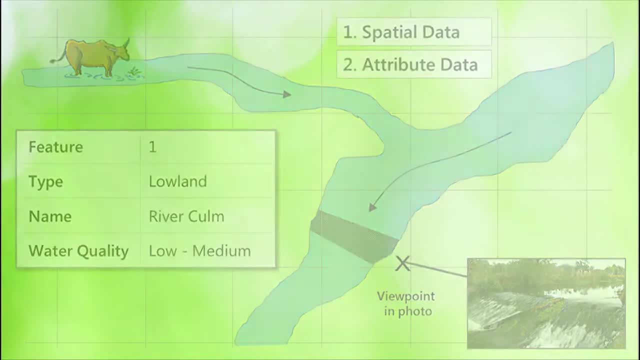 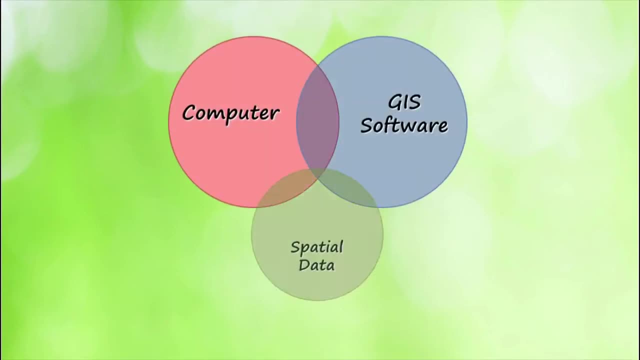 And so we can begin to gain an insight into how the ecosystem is functioning. So what exactly is a geographic information system? Well, a GIS is actually comprised of four critical components. The first three of these are a computer, a software application and a collection of 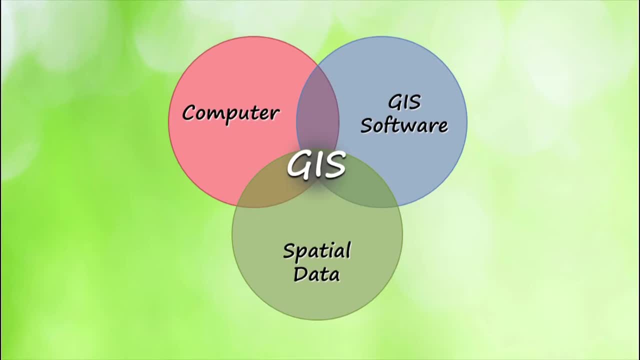 spatial data, While the fourth, and perhaps most important, is a data collection system. So what exactly is a geographic information system? Well, the first and most important component is the user. It is the user who needs to answer a spatial question to produce some spatial evidence. 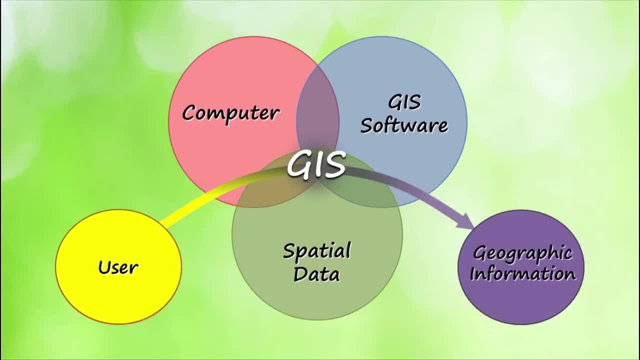 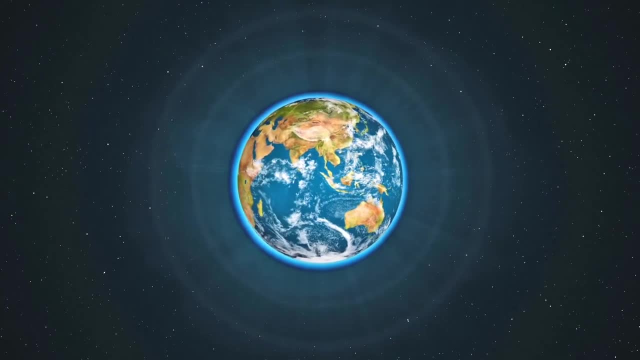 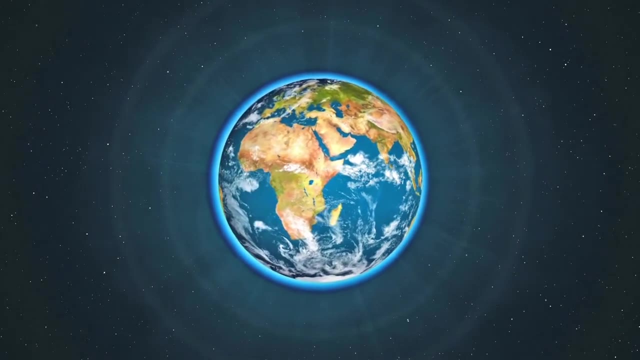 or to communicate a spatial message, And it is the user who has recognized that a GIS is the right tool to achieve this objective. Before someone can become a skilled user of GIS, it is, of course, vital that they develop a technical understanding of spatial data and how a GIS application can be used to interpret. 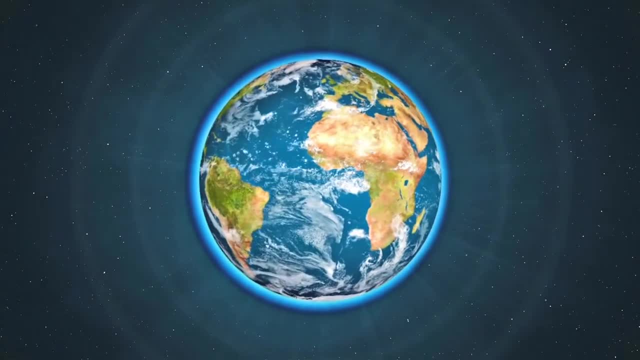 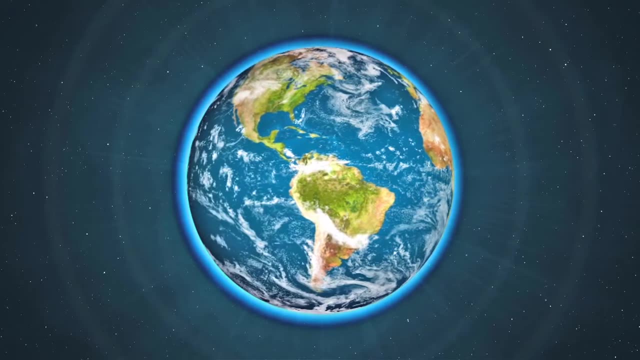 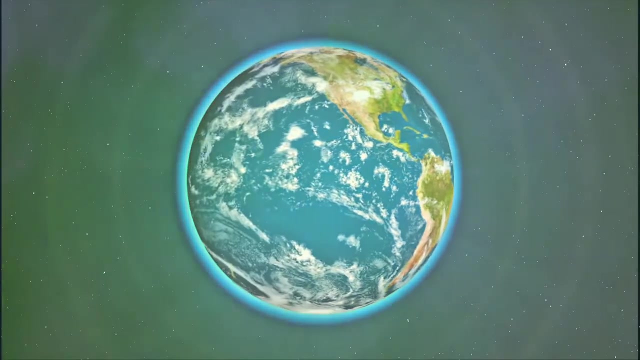 and interrogate that data. However, before these technical skills can be used, it is perhaps even more important that they first learn about the different ways a GIS can be used to produce different types of geographic information. Otherwise, how can they recognize when GIS is the tool they need to use? 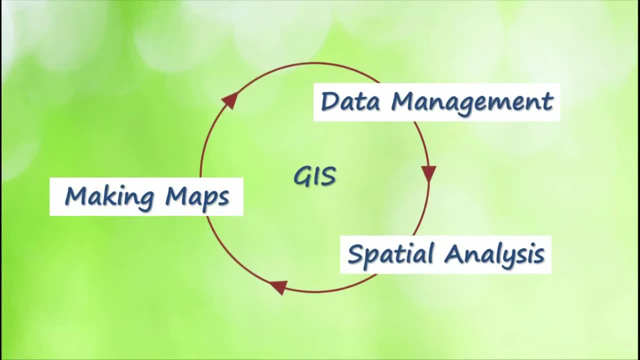 The application of GIS falls into three broad categories. A GIS provides us with a powerful tool for the creation and management of spatial data. A GIS allows us to answer spatial questions And to perform spatial analysis And to perform spatial analyses on the data.